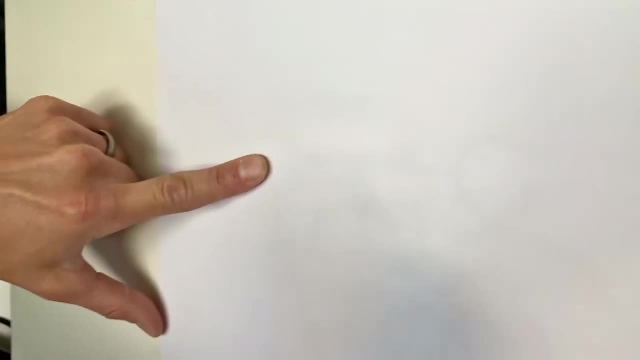 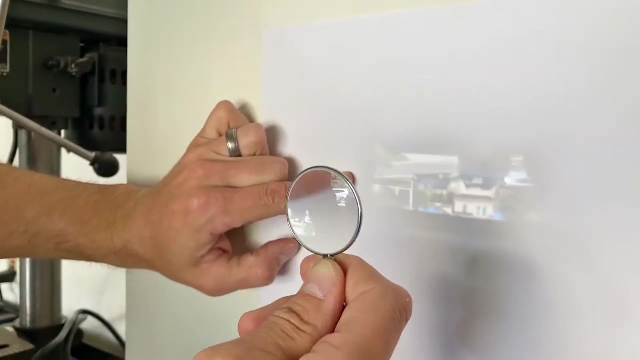 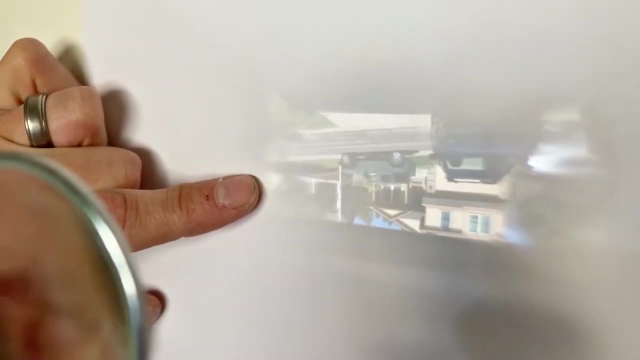 focuses and we get an image on the wall. If the lens is too far away, it's out of focus. The light is passing through here, but it's out of focus. But when this is just the right distance away, this image forms, And that is what we call a real image. You'll see. 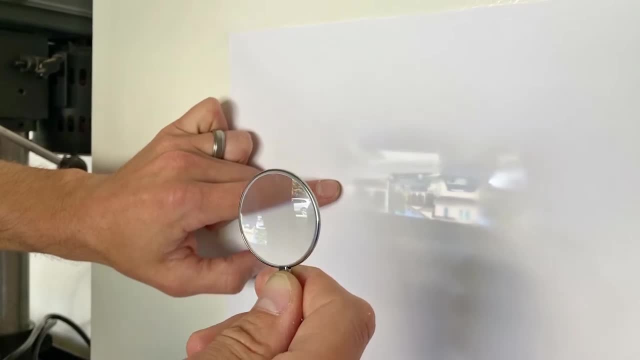 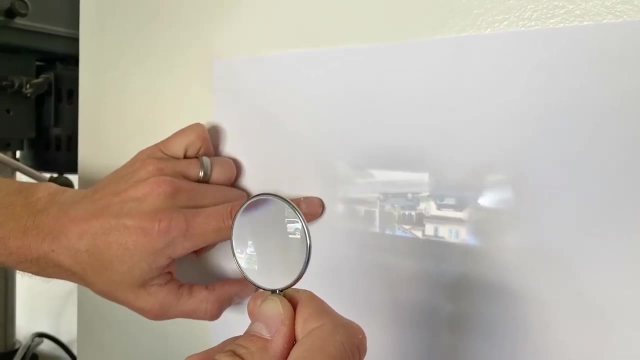 It's inverted and it's smaller and it's out of focus. So when you take the focus, as I've, you can do the math for that. you can see that in some of my other videos for convex lenses. you'll see what we have here is a real image. we say it's real. 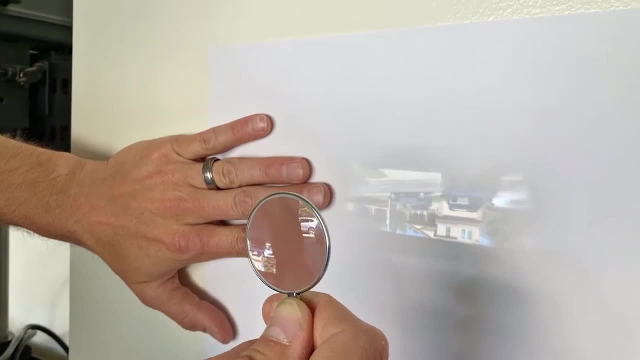 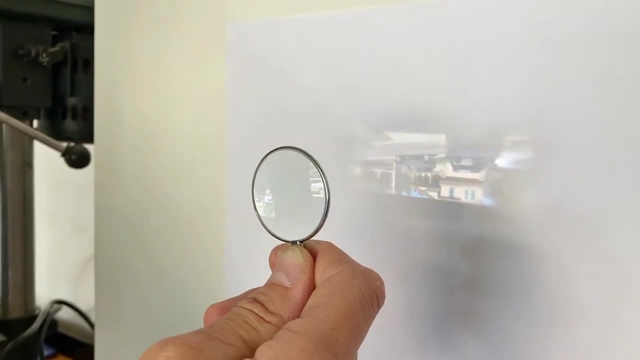 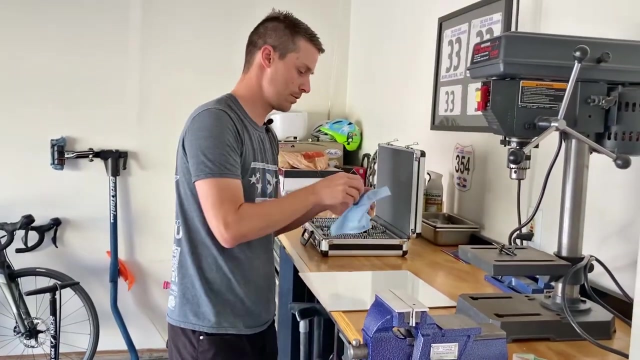 because it can be projected onto a surface, or really it's. it's real because the image is on the opposite side of the lens, from the objects, in this case the car that just drove by now. we can do the same thing with a mirror, so here's a. 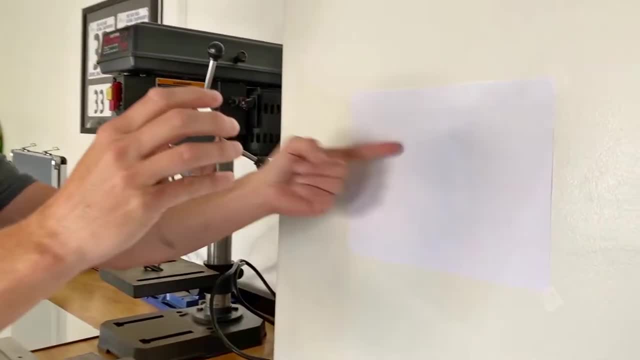 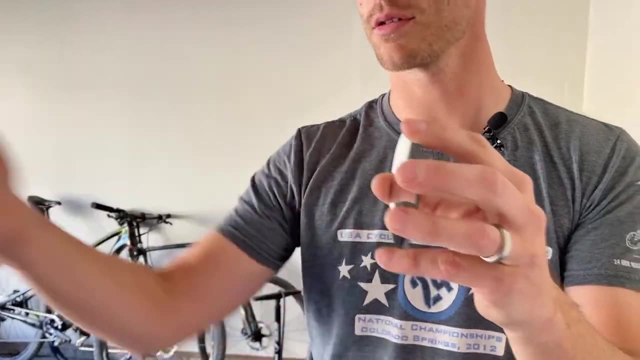 mirror. this is a concave mirror. now, if I try to hold this up against the wall, it's just gonna reflect a wall. now, if I hold this so that it's reflecting light off of what's outside, you'll notice there's nothing for this light to. 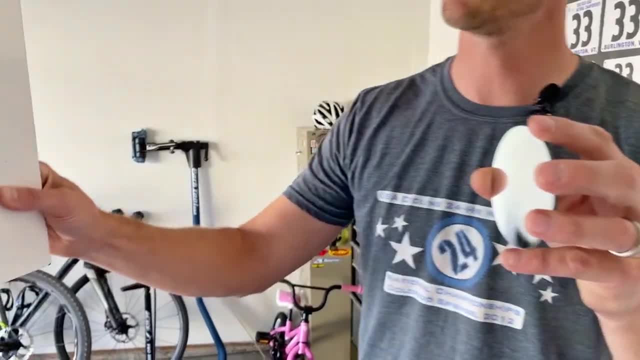 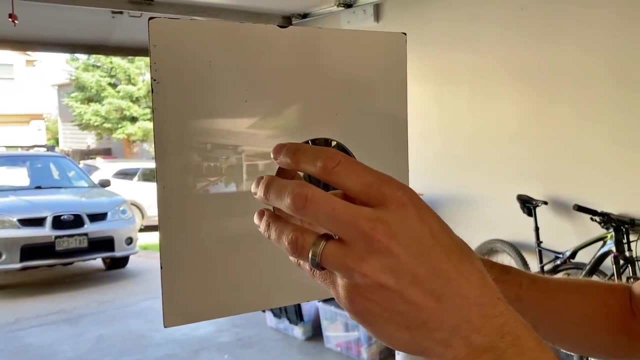 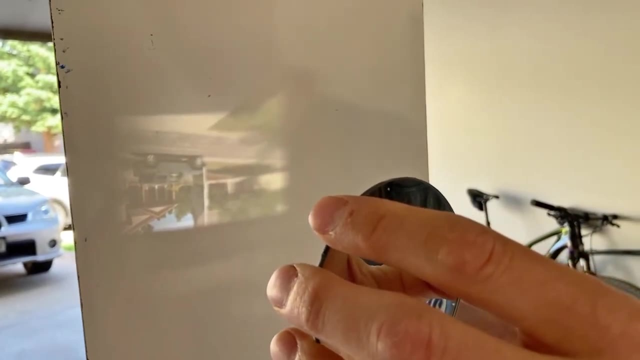 project onto, which is why we got a whiteboard. come around over here just see. this mirror is projecting an image onto the whiteboard would say that's a real image. that image appears on something we can project it onto. now, in the case of a mirror, a real image. 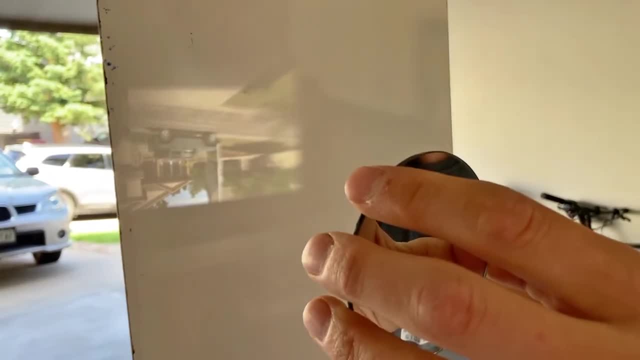 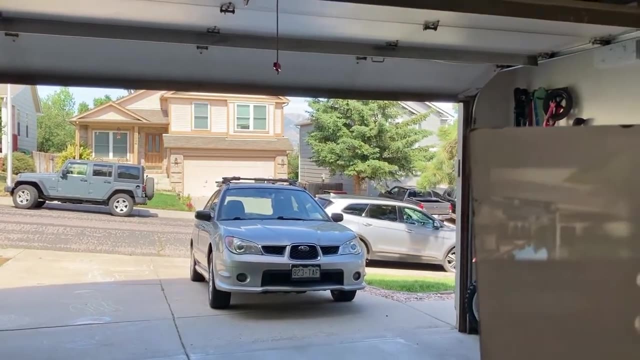 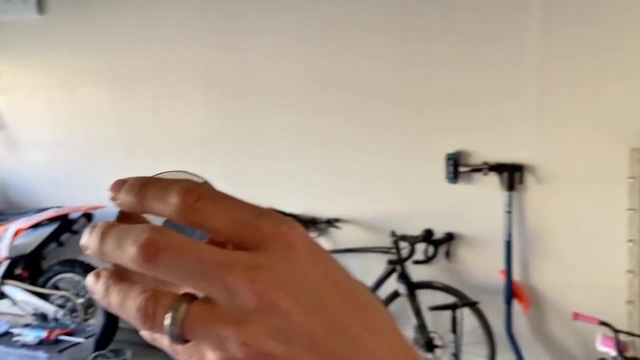 shows up on the same side of the mirror as the object. in this case you've got the Jeep in the background and then the image of the Jeep sitting against the whiteboard. now the question comes up then: what's a virtual image? if a real image gets projected onto something, stay right where you are. okay, now you're. 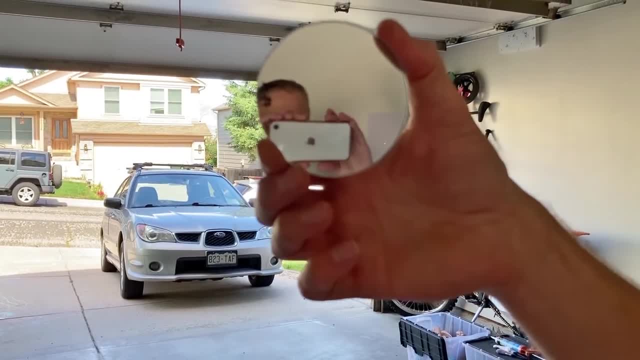 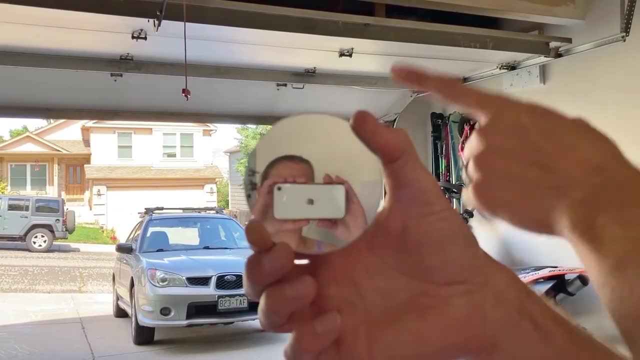 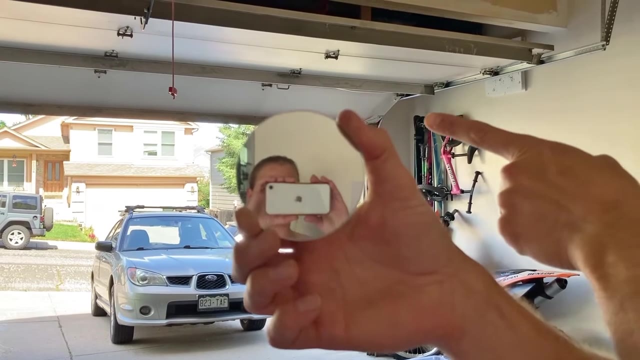 looking at a virtual image of my wife trying to videotape this. can you see you in there? so what you see is an image that appears as though it's somewhere back here. it appears as though there's a teeny, tiny little wife inside my mirror that is recording everything, and we can see a.